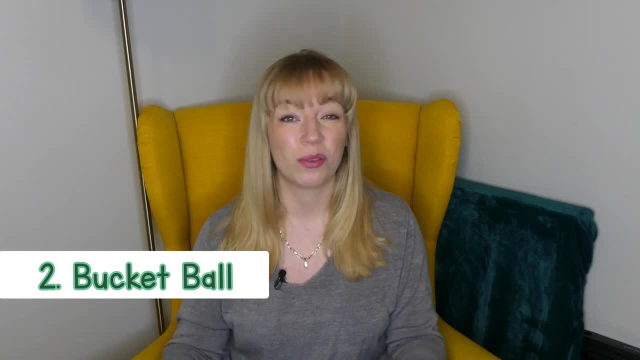 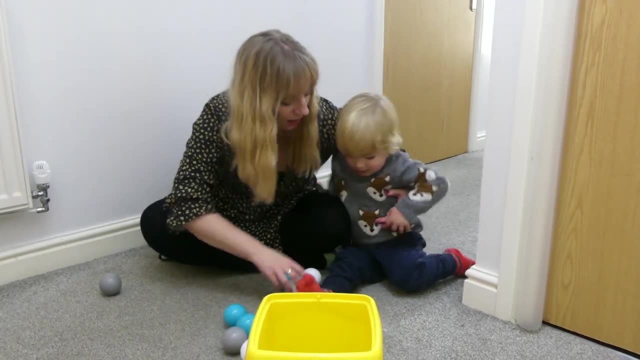 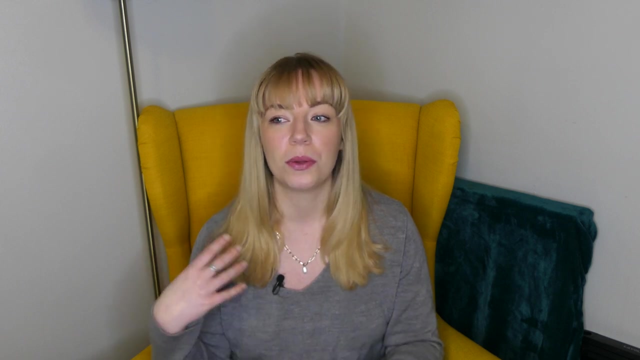 easy to play. So if you're going to use a bucket or a box or something like that and some balls, you're going to throw them in and at the end of the game, when you've used all the balls, you can look in the bucket and count how many landed in the bucket. So this is that one-to-one. 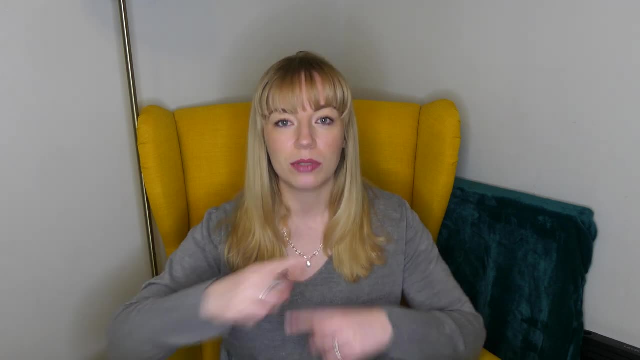 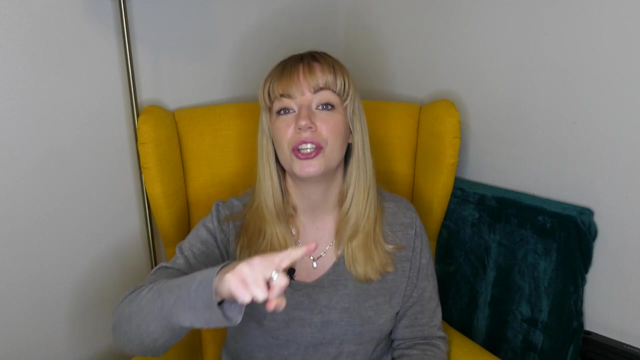 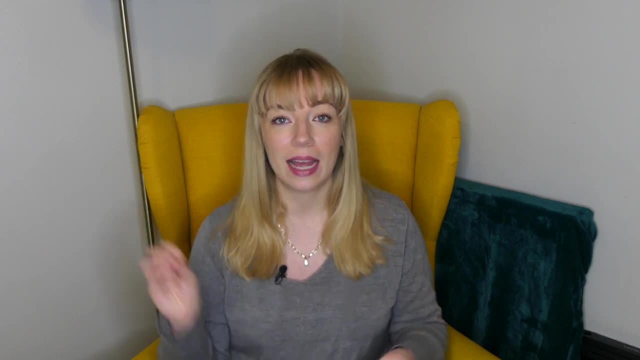 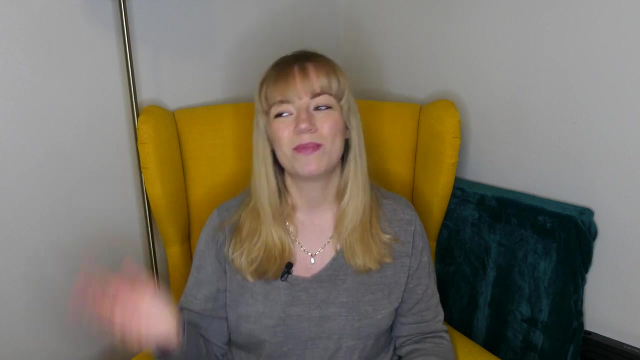 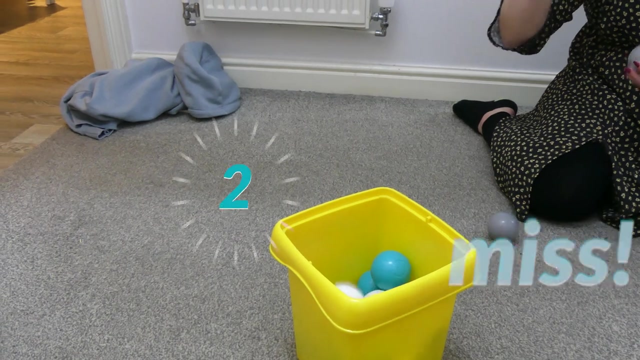 until you've put your finger on the next ball. You can also play this by counting as you go, if you think your child's ready for that. So if you get one in one, Okay, I got one in. Didn't get that one in, I got another one in, That's two. You can also make it competitive and have scores going on. 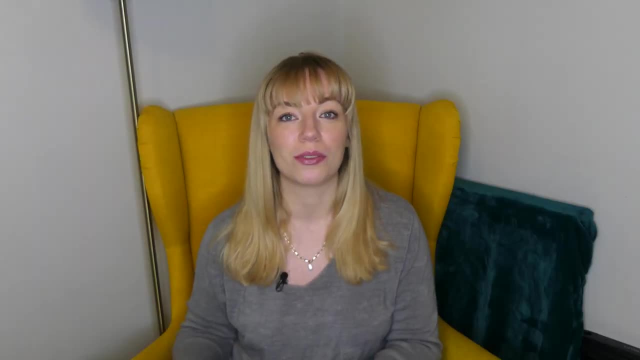 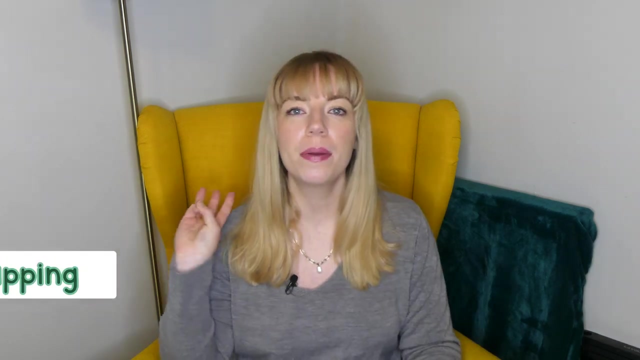 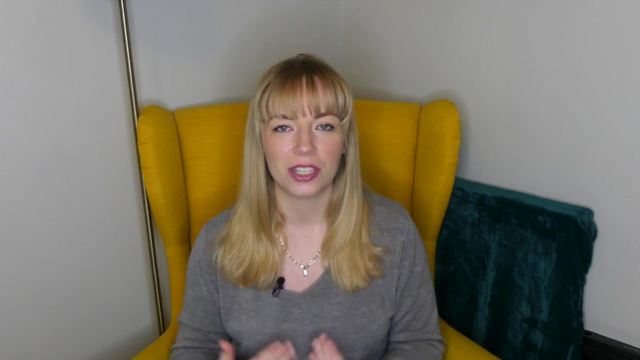 and really just make this game your own, depending on your child's age, stage and ability. Just as a side note, my son is two and he loves this game. Number three: clapping Or other things I'll explain. So it's really important when children are learning to count. 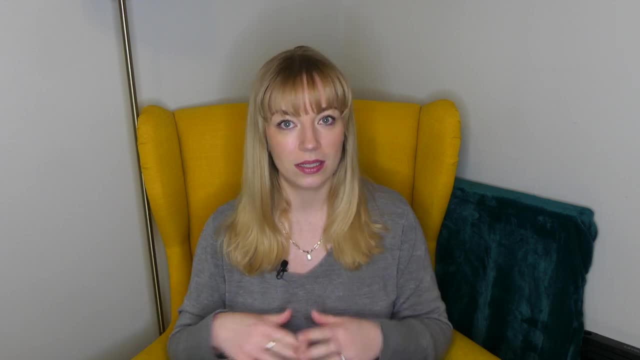 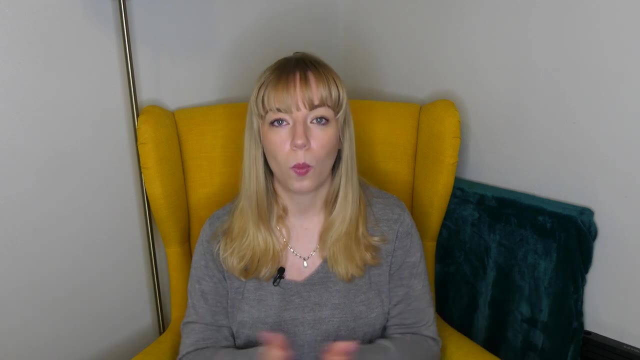 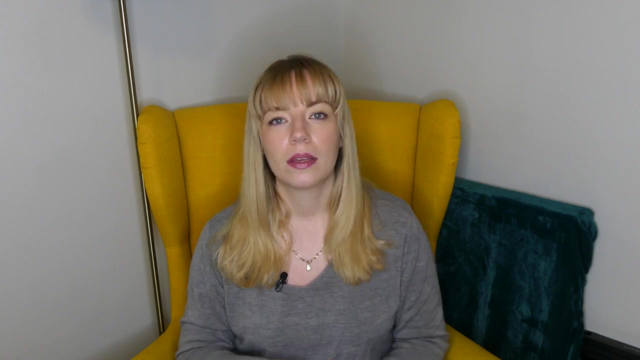 that they know that it's not just objects that can be counted, it's pretty much anything. So we can first start doing clapping. So listen to my claps- One, two, three- And have your child then repeat it back to you- One, two, three, As they get more confident with that they can. 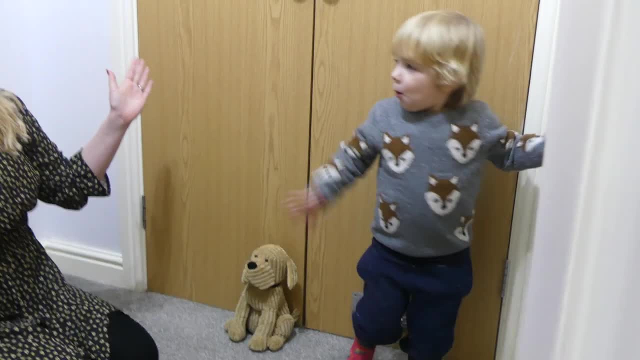 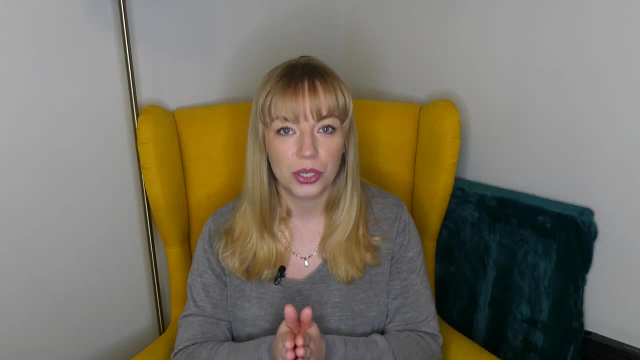 start clapping to you and counting their claps- And remember that it's that one-to-one correspondence again, so not counting until you've clapped. So one, two, three. You may find that some children start doing something like this: One, two, three, four, five. 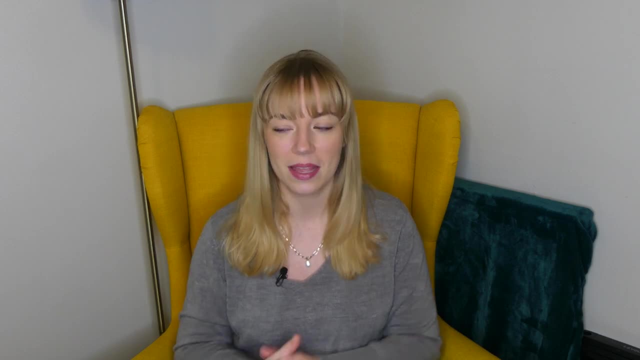 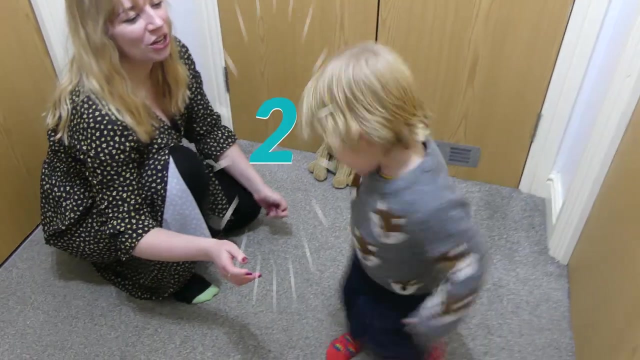 six. So there's that one-to-one correspondence coming in there, And you can also do something else like jumping or spinning- although be careful with that one Stomping making noises. anything you really like to do, that doesn't involve an object. You can really just. 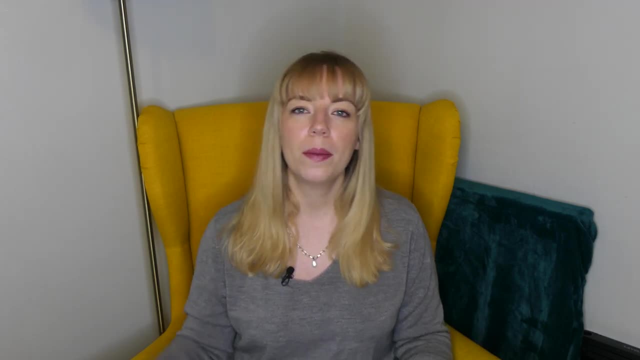 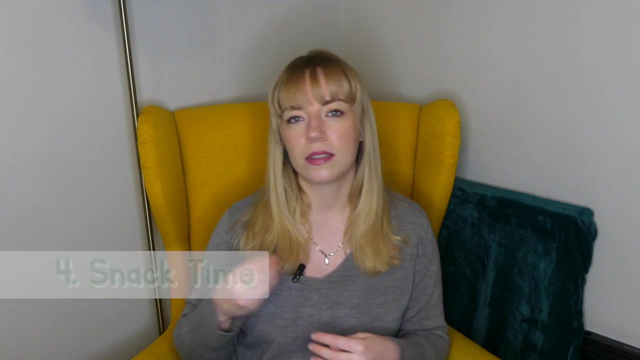 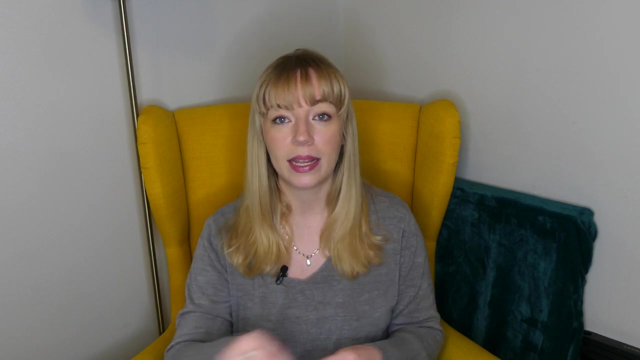 get creative with this and then be counting as you go along. Number four: snacks. So at snack time, if a child is having something like raisins or some breadsticks, something that they're having more than one of, you can count with them how many you've got. Maybe they get four and you get.